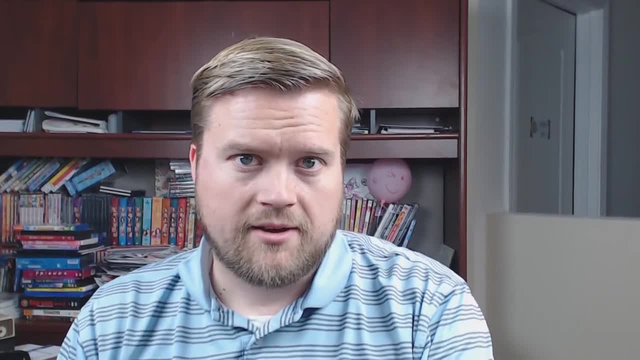 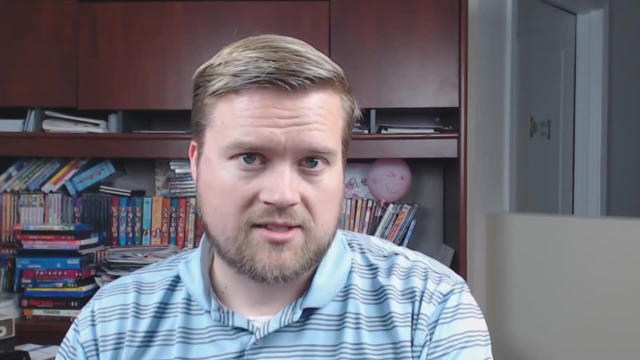 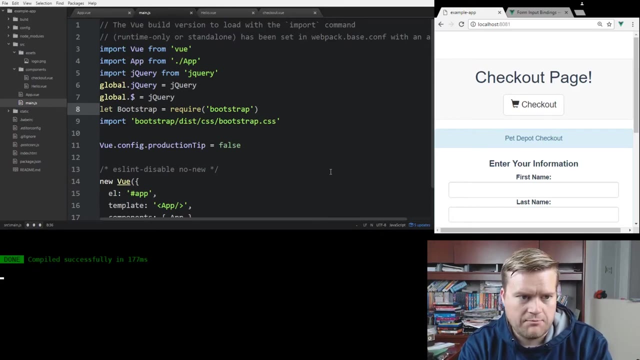 your favorite frameworks, including Aurelia, Vue and Emberjs, and I also do developer interviews and I give advice. So if that's what you like, please click that subscribe button. Now let's begin. Hey, so last time we left off, we had added Bootstrap and jQuery to our Vue app. 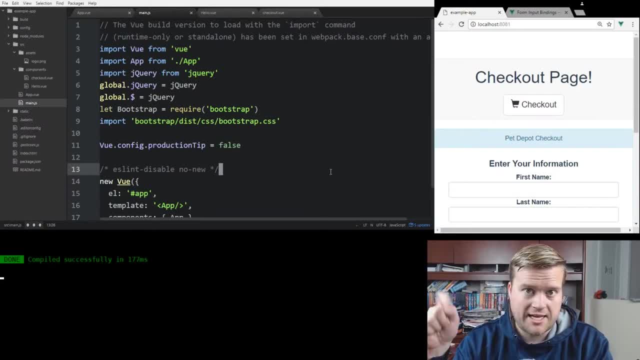 If you are confused, then take a look at the playlist I have for Vue. In the last previous video I created an app with Bootstrap and jQuery, So you can see here on the screen this is how I did it. Now I went ahead. just for time's sake, I went and created a Bootstrap form. 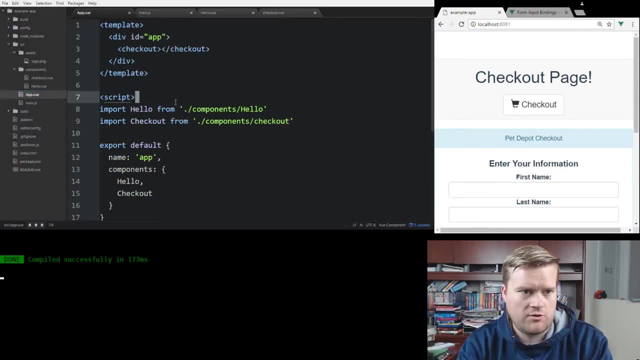 for us. So let's take a look. So if you look at appvue, I created a new checkout component and I went ahead and imported checkout from component checkout, which is here and you can see here in the directory structure here, And I went ahead. 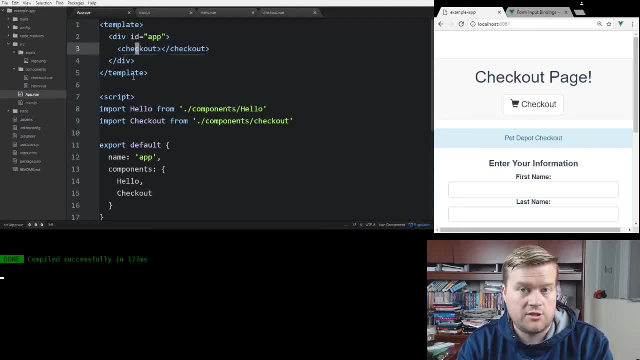 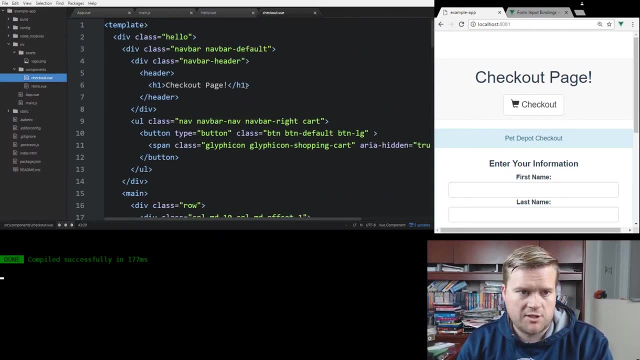 and deleted out the default hello one in there and just made sure checkout was in there. Now, inside the checkout component, I went ahead and used some form groups and I used some Bootstrap to create a checkout page. It still has div class hello here, but it doesn't really matter. 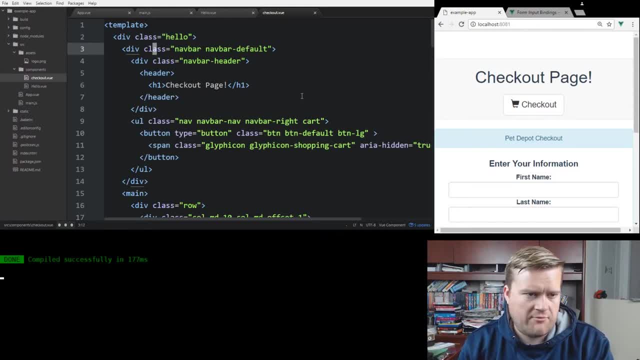 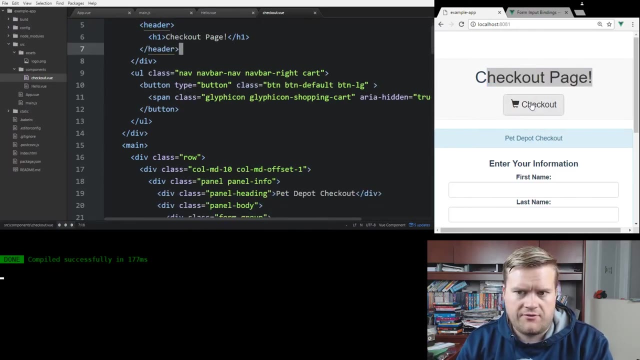 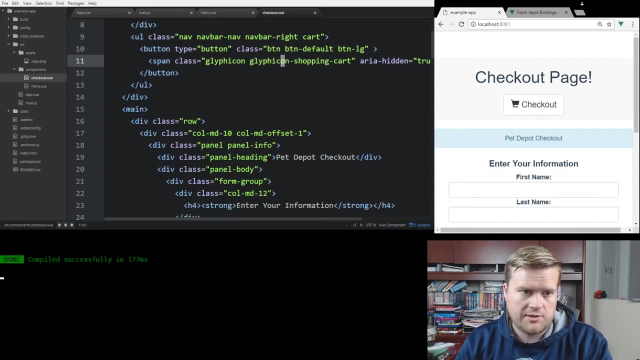 And inside this div class I have this nav bar. you could see here I have this nav bar and inside the nav bar I have a header that just says checkout page. you could see here. And then I have just a little checkout button using the graphic icon that comes with it, And then inside, 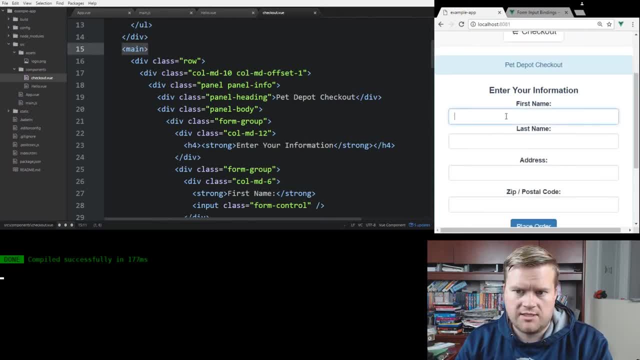 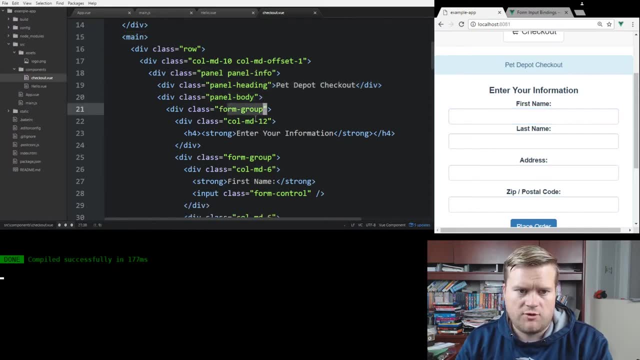 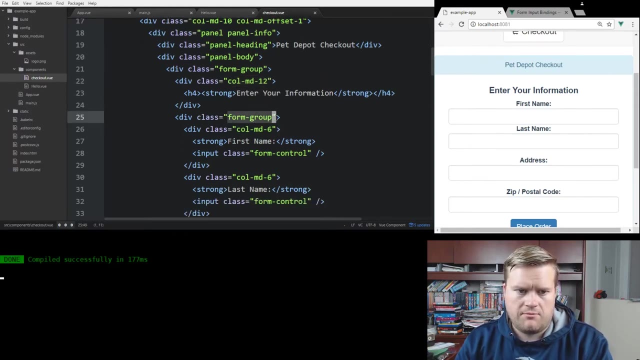 our main here. I have a few rows, and each row is a different column, a different button here. So I have a panel heading, panel, body, form, group, and then I used the grid layout with the column middle: 12.. And then I use six and I have a first. 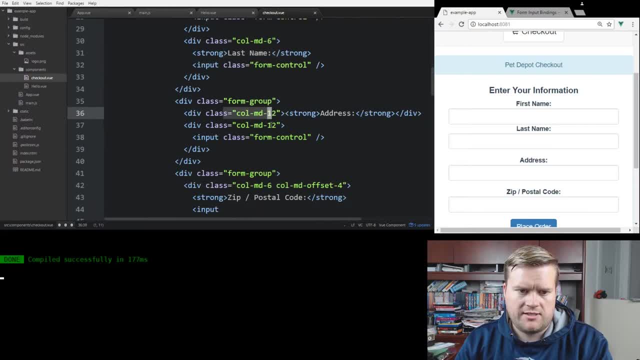 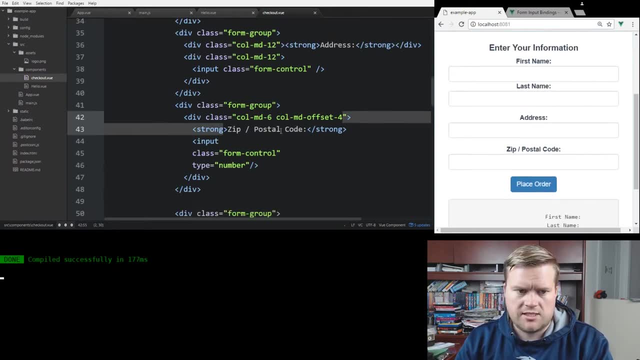 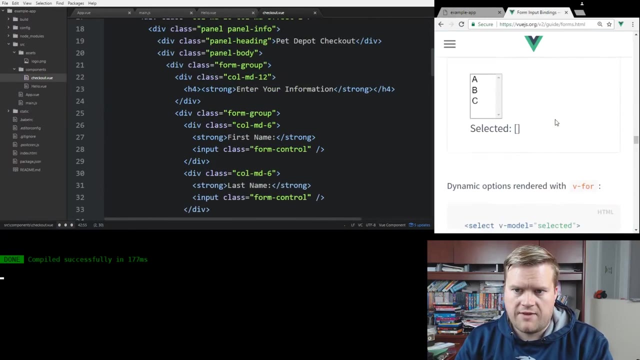 name and a last name and an address and a zip, And then underneath here I put a pre, just something, so we can see the output of each one of these. So, if you don't know, there is something called a V model and the V model, it allows us to bind. 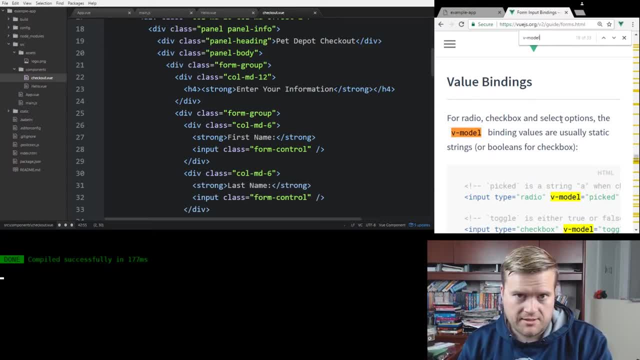 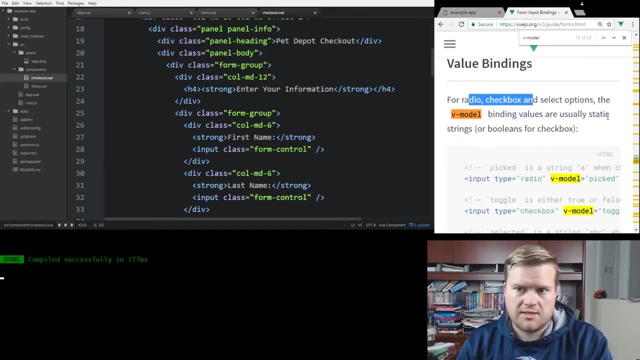 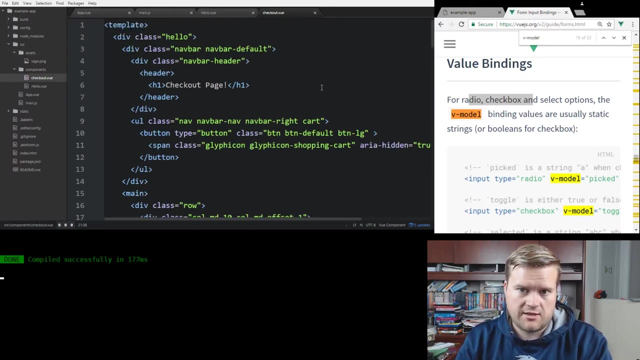 do a two-way binding in our template to one of our input form controls So you can put it on radio button check boxes and select options. Right now we're just going to do a normal input text box, but we have. we can do it for text areas and other things as well. 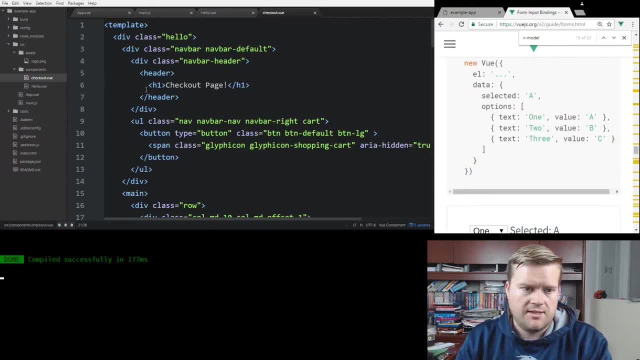 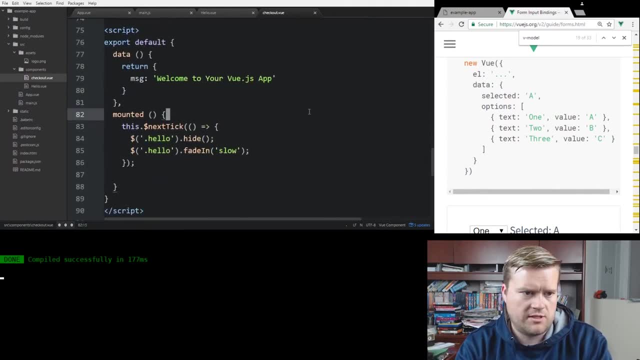 And you add components too, for that matter. We can show that later. So let's take a look here for first. If we go back down, we could see- here's our next tick- where we had the fade in. but we do have our return object and I guess we're not really using. 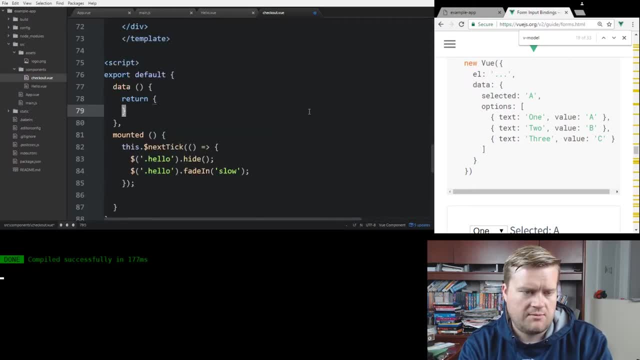 the message are we? Yeah, So we can delete the message, but let's create a checkout object And this object's going to hold all our values, So we can do something like this. We can call it. well, just for the sake, we're going to call it order and we're going to make. 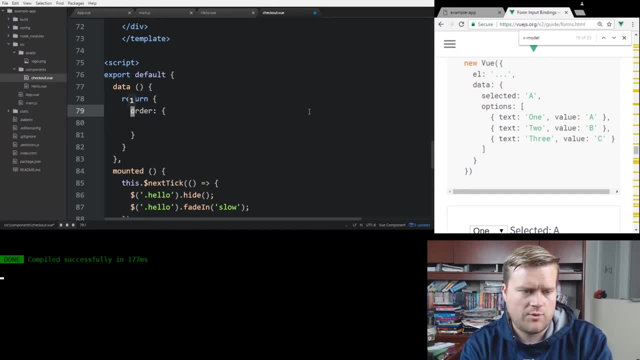 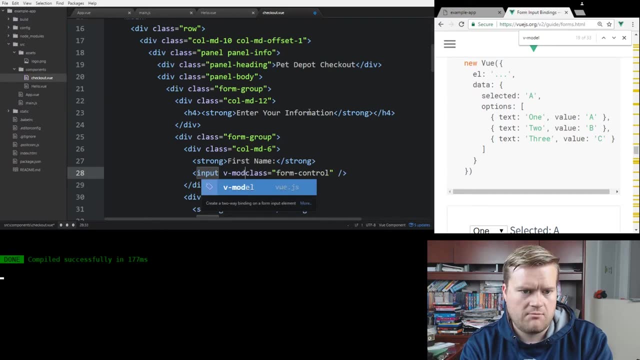 it an empty object for now, And then what we can do is we can go back to our input- Here's our first name- and we can use the V model, the V model directive, and then we can name, put it the name of the object that we just created. So let's do object or let's do order. 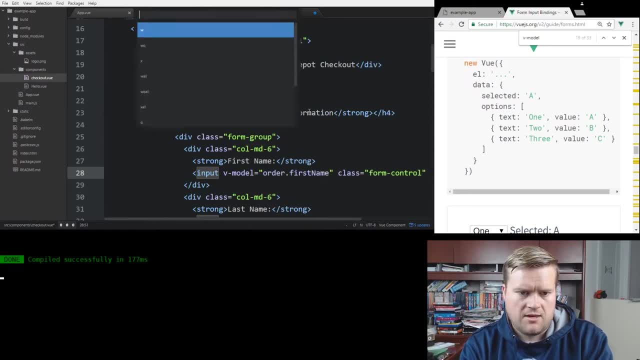 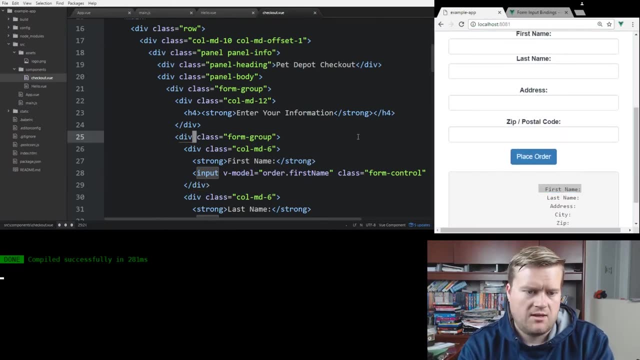 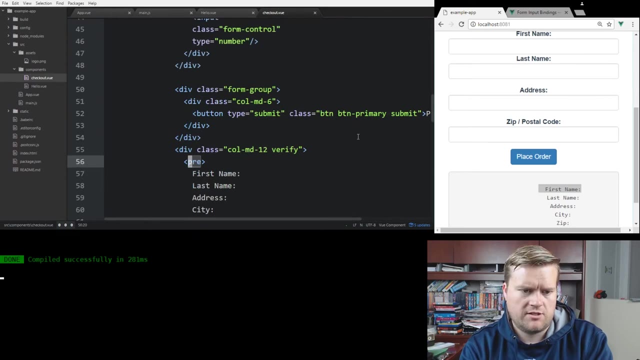 dot first name and compiled. Okay, Still, we don't have anything here in our first name box. So if we go back down, let's go back to the pre. So here's our first name in this box here. So let's go ahead and remember: inside view: you have to have these double curly braces and we can. 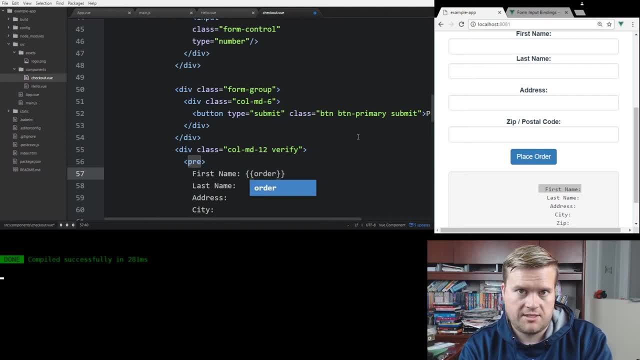 put in a name of one of our properties and in our data object. So we're going to do order dot first name and we're going to save it So you can see here, right here I have a first name and I can type stuff. 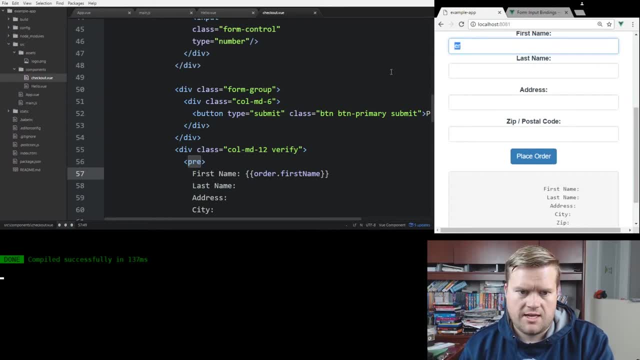 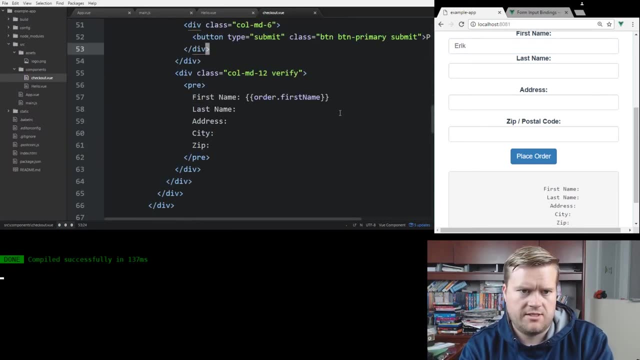 Let me refresh it. and we don't see anything, So wonder why? So we can go back down here to our order object and we see that it's just an empty object. but let's add a property here. So let's add first name and we'll save it. Now let's type something. Okay, Now you can see here. 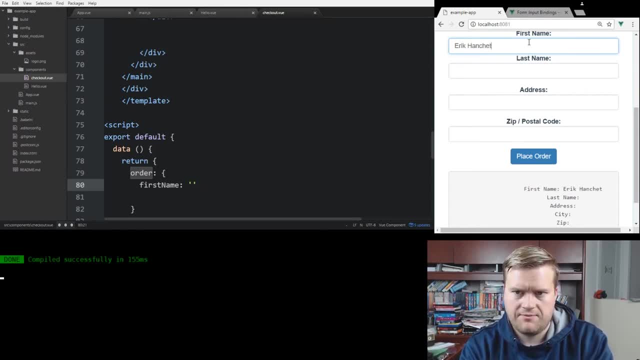 as I type it, it's being added in here. Excuse me, Eric can't chat. So this is what's called two-way data binding, because as I'm typing this, it's being updated in the template in the same time- real time. So they are hooked together. So let's go. But one other thing we can do: 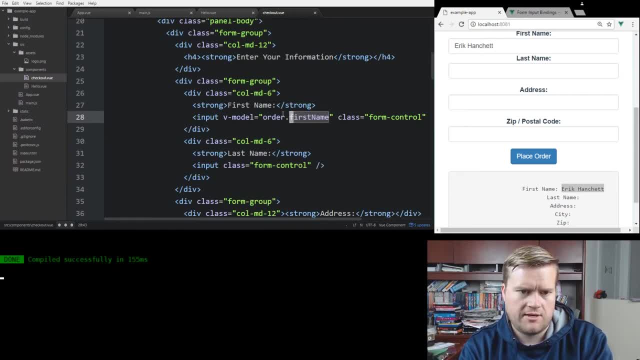 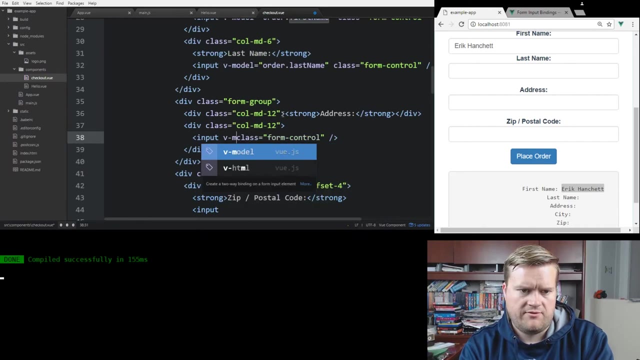 Um, so we have this order dot first name. here We can. let's go ahead and add a couple more. We're going to add one here. We're going to add a v model. Let's do order dot last name And for the address v model, order dot address. and when you 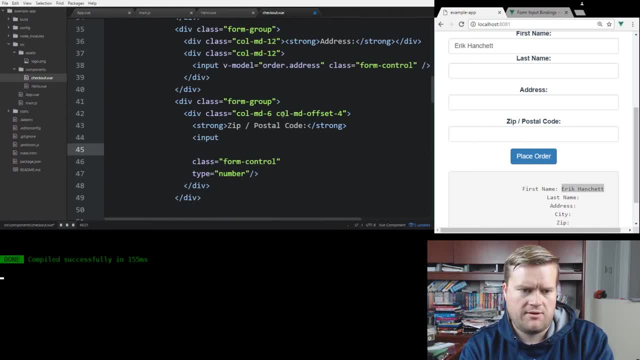 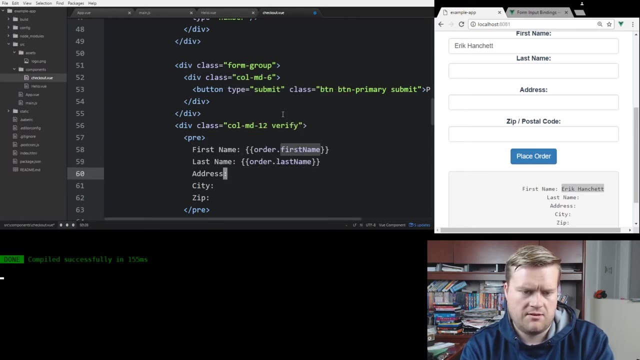 can name these whatever you want, and right here I'm going to put in a v model, order dot, zip, and then inside here we're just gonna put those in here: order dot, last name, order dot, address, order dot. well, we have sitting here. we don't have a city, but we do have a zip. 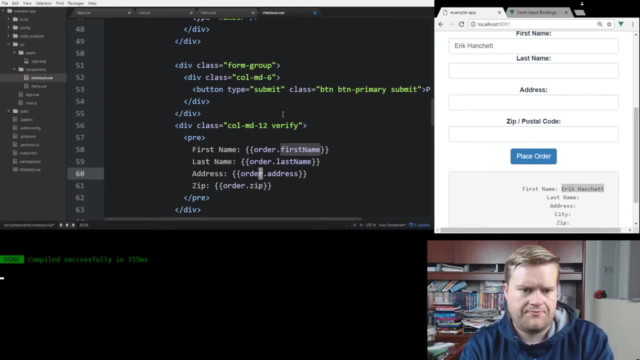 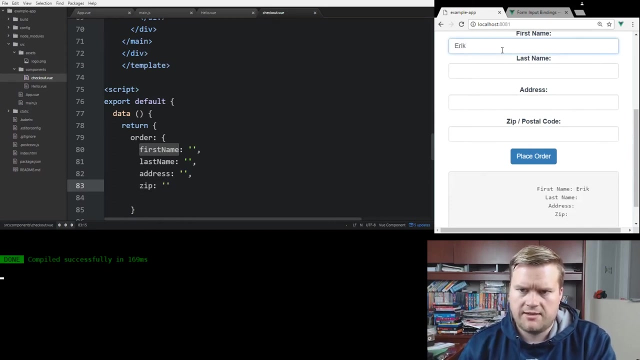 order, dot, zip. okay, so we have them all in there and let's just go down here. and, to be explicit, we can go ahead and add all these in here. so we have last name. we can also put default values here- address and zip. so we'll save it now if we type in the first name. you see that. 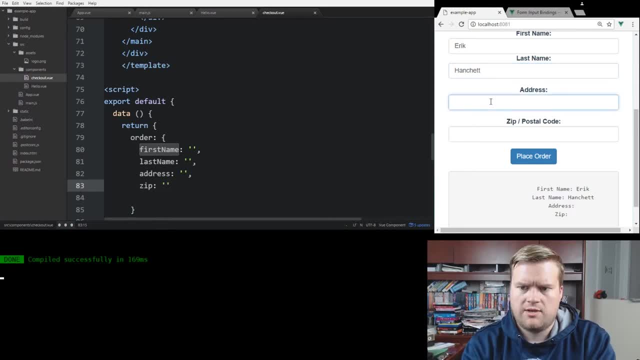 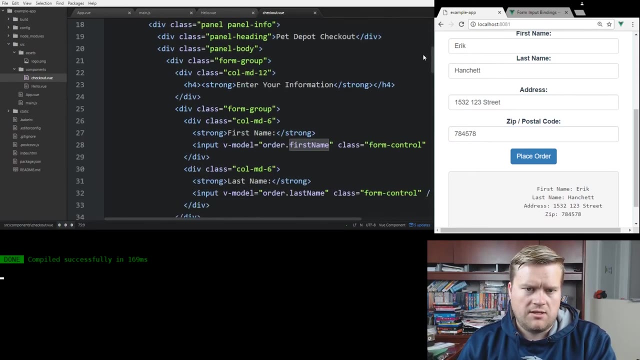 type in the last name, same thing is updated, the address 1532 123 street and we can put it zip code 782. so everything's being updated in real time there. it's always two day data bind, uh. another thing we could do is in this first name we actually 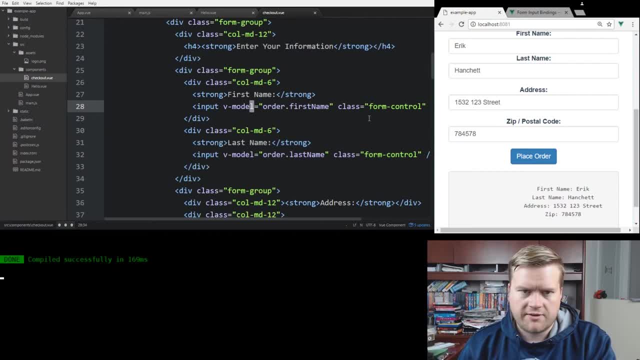 have some modifiers that we can use. so there's three modifiers that we can use with the vmodel directive and they are, if i double check here: uh, dot, there's dot number, dot trim and dot lazy, so let's take a look at the first one. so if we can go, 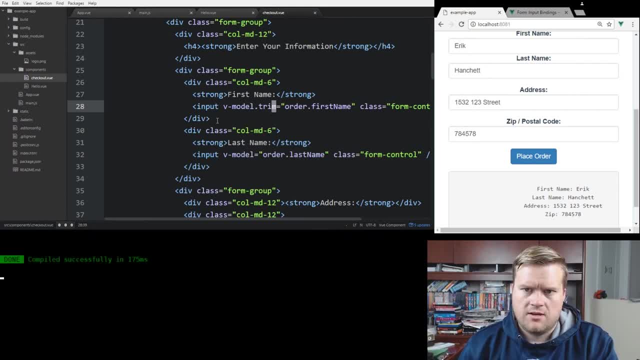 vmodel dot trim and we'll refresh it here. so if we type in like a bunch of spaces and type in eric, you could see down at the bottom of the screen here that you don't have any spaces here. it's out automatically trimming it. i mean you can do hand chat here. you could see in this one we don't. 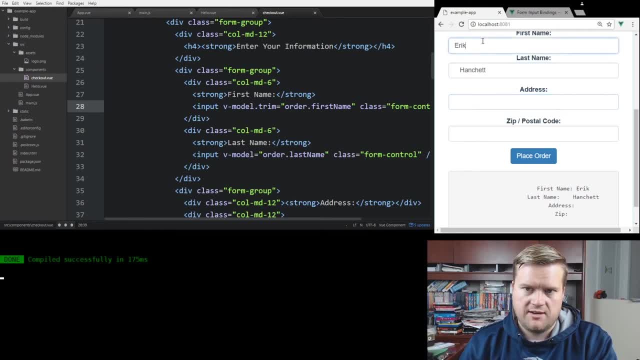 have the dot trim and then we can go vmodel, dot trim and we'll refresh it here. so if we type in a trim and you see a big space right there, but in this case if we put spaces before or after, it trims it, which is really handy. so that's one of the modifiers that you have, vmodeltrim another. 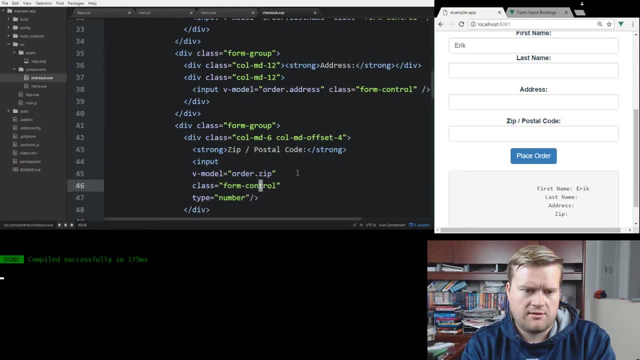 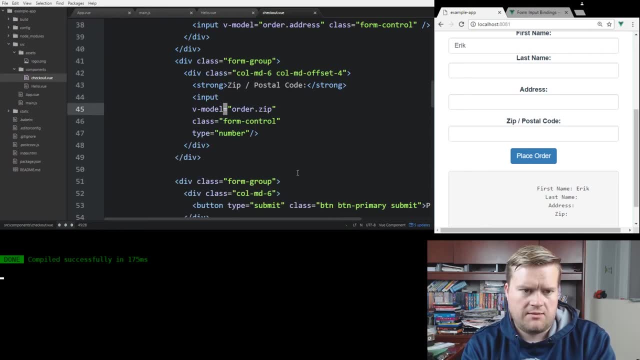 let's say, is vmodel. we can go to the zip. it's vmodelnumber and what this does is, by convention, all these inputs usually come over strings, but by putting a dot number it comes over as a number. so if we put in a number here, of course it works. 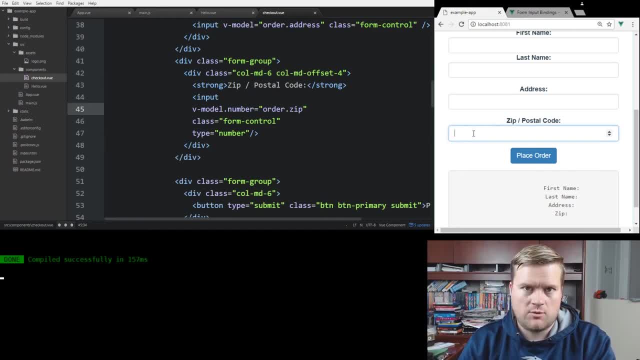 i'm typing in keys here and it's not working because it's expecting a number, even though we have type number here. so let's delete the type number just to see what it shows if we don't have that in there. so so so since we have, we can type this in. but if we do eight, nine, five, two, three, 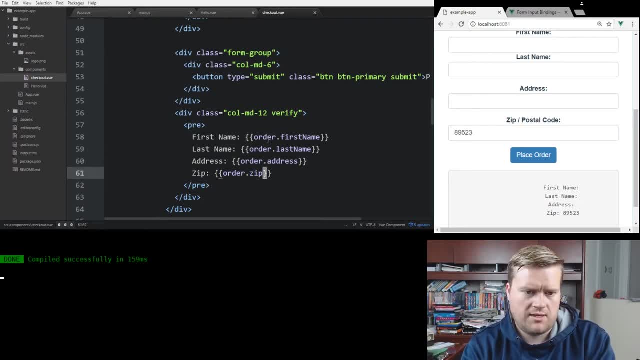 and let's go back down here and let's do the javascript type of, and so you can see, here it comes over as a number. obviously, if you put a string, it comes over as a string, but if you put a number it comes over as a number, which is what we want, so we don't have to. 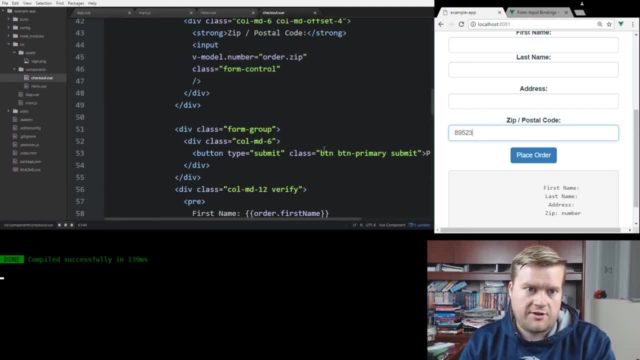 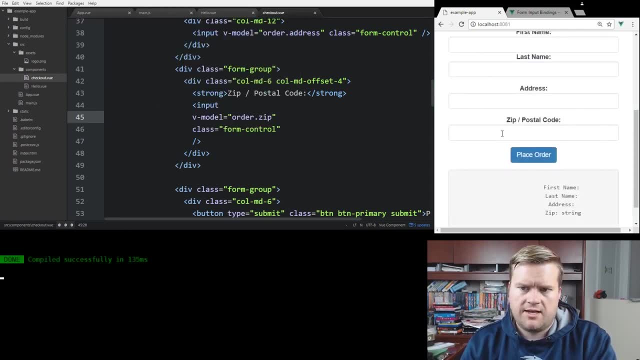 do any kind of type of conversion inside our javascript. on the other hand, if we didn't have this dot number here, i could show you we'll save it and we start typing in here a number. see, it always comes over as a string. you can see here it says zip string. so that's one way of of doing it. 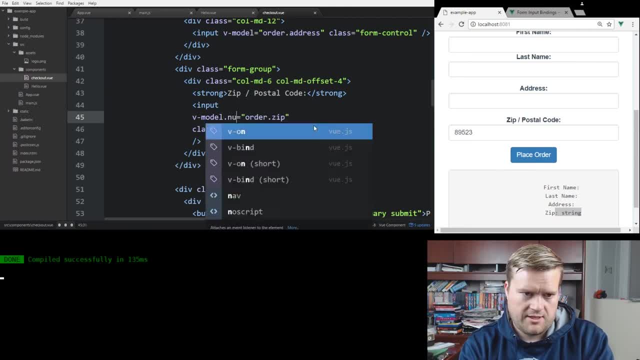 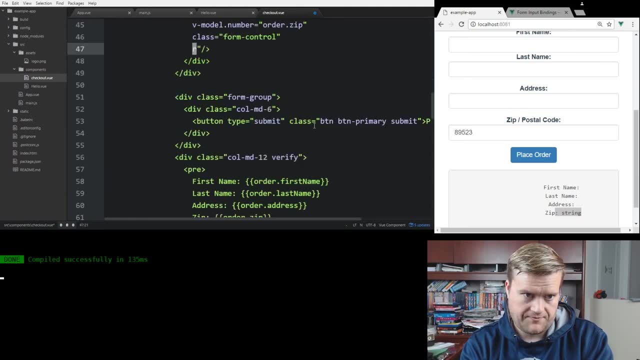 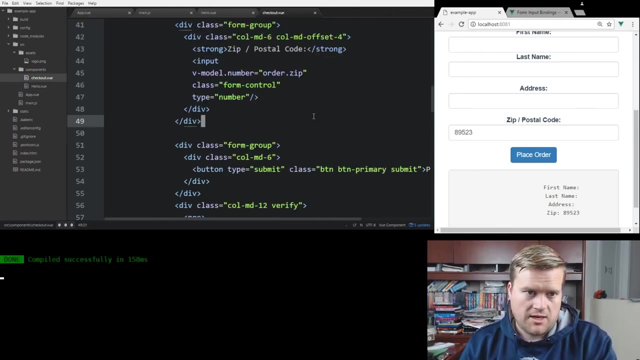 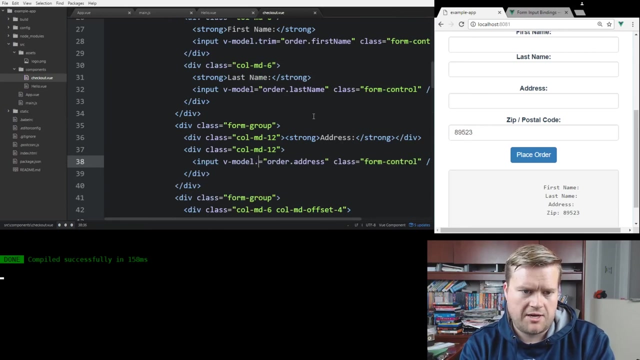 so we don't have to worry about here we can do this. type equals number, so that's one way to do it. you can guarantee that it's a number. and then the last kind of modifier is dot lazy, which changes the, the way it binds. so if we do dot lazy here to this order address. 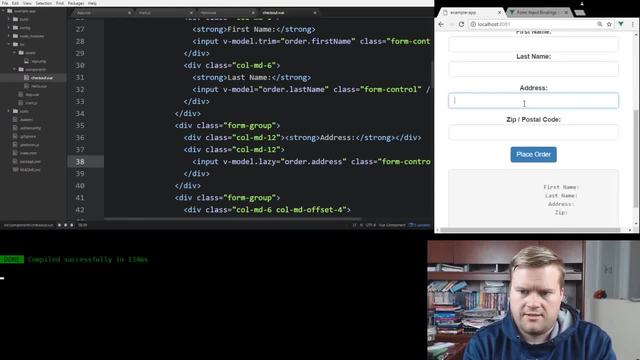 refresh it and if you see i'm typing here, it's not automatically syncing one, two, three street, but if i click out and i lose focus and then it updates, so it changes the time that it updates um to to some time later. so that's, that's pretty handy. 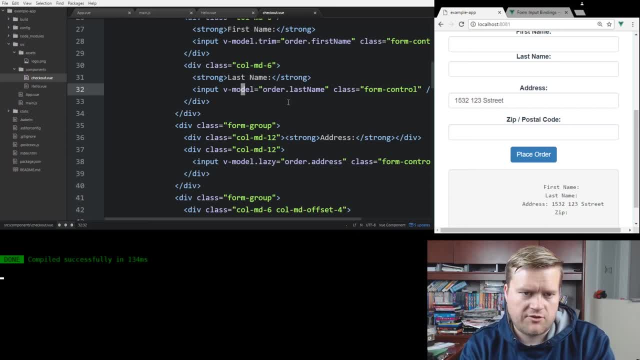 this actually um. those are the three main ones for v dash model um. if you're thinking about one-way data binding there, there are ways of doing that um by default. if you're passing in stuff into components, the it's, the properties go in. they're immutable. uh, they actually um. 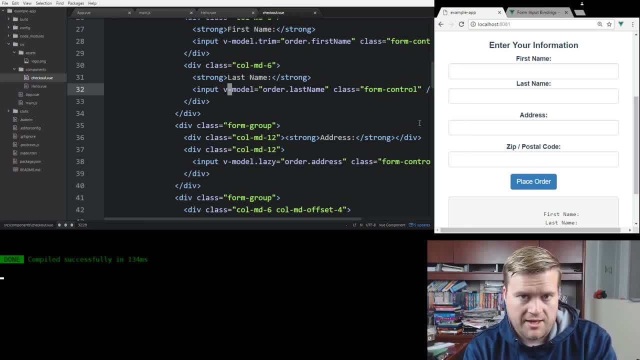 the convention is is that you send properties in and then you send actions back up to change those, so you don't necessarily change them. it's not supposed to be two-way data binded. um, there's also something called v dot once, which is another way of of doing two-way data binding. you can see here i'm typing in: 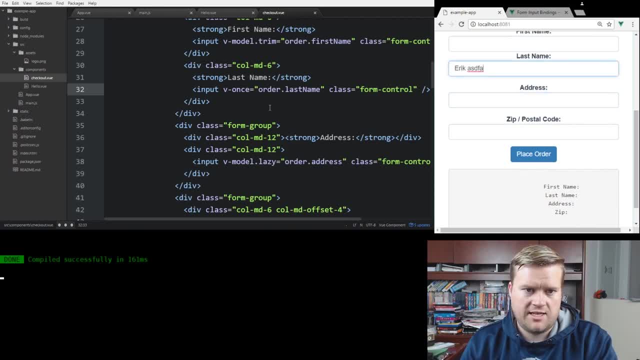 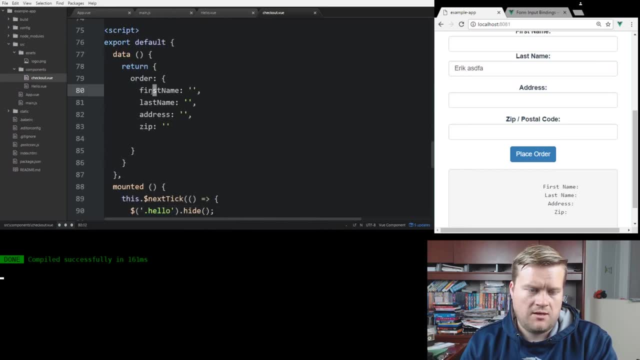 a name and it's not being reflected down there because it only binds it once. so if we went back to order dot last name, here at the bottom we can put a default value. um, actually that doesn't work either. yep, you can see right there. right there, it bound to. 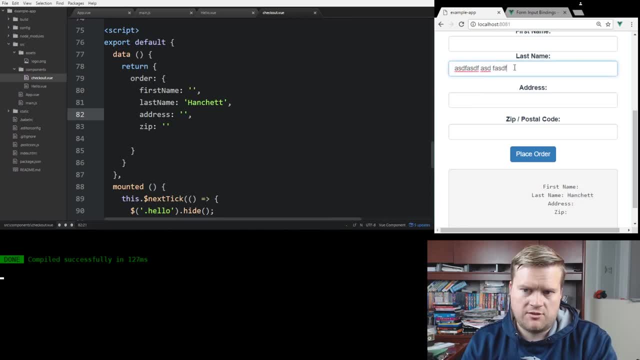 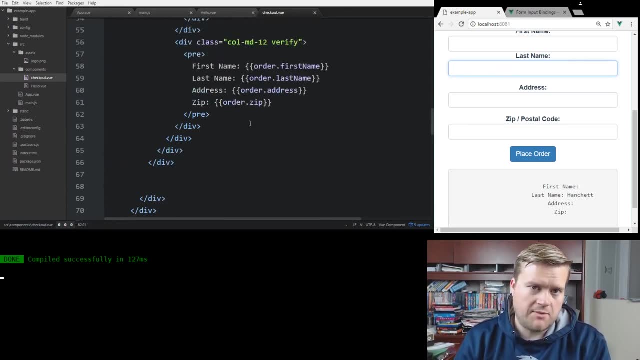 hand chat, but if you change it it's not going to automatically update or anything like that, because it's kind of one way. so those are just a quick few things on the v model directive in v once. on the next videos i'll talk a little bit more about that in a little bit more detail, but i'll